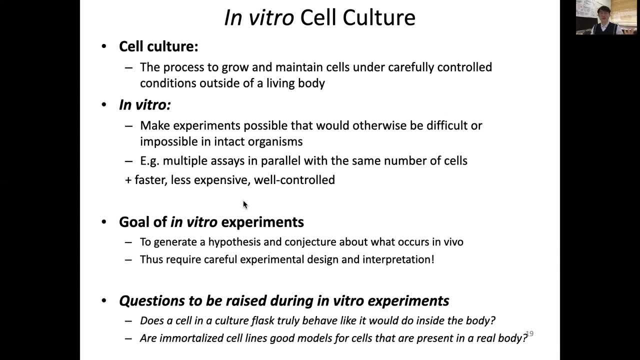 And conjecture about what occurs in vivo, which is the most important in the end. So what is hypothesis? Hypothesis is a worldview that is testable, So you can generate hypothesis, which is easier with in vitro experiment, And that clue can be bring into in vivo and hopefully, maybe a human or clinical practice. 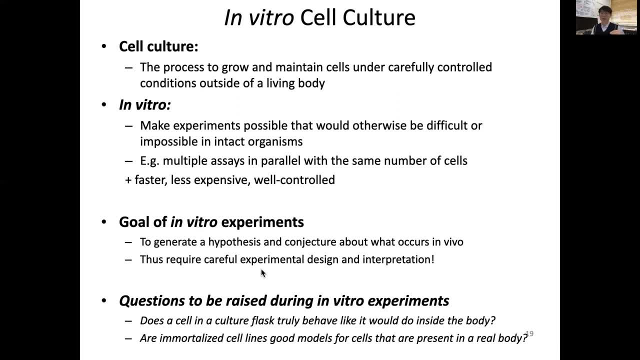 So in vitro experiments require careful experimental design and also proper interpretation. So we have to keep in mind that during this in vitro experiments we have to ask ourselves that: does a cell in a culture flask dish truly behave like it would do inside in the living body? 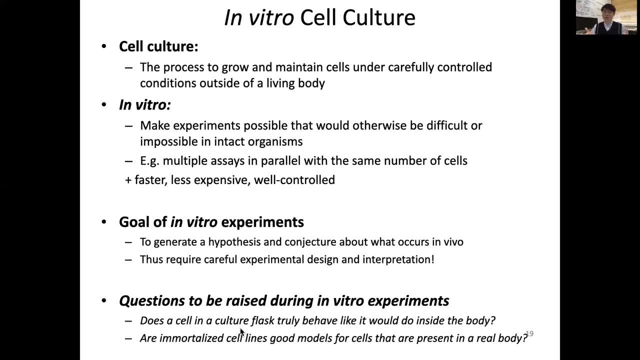 And many times in vitro experiments we use a cell line which is a neutral line And many times in vitro experiments we use a cell line which is a neutral line. So in vitro experiments we use such a design that there actually exist certainly. 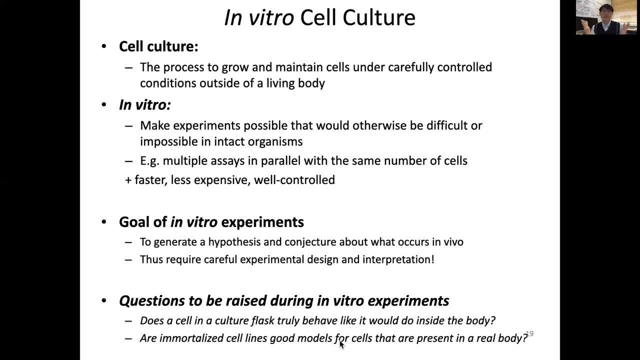 there's noicy cell lines with neutral lines. So we say how do we see our in vitro evidence? And if we say Let study, Let's say look at some samples to the in vitro experiments- cancer or cervical cancer- from decades ago, from one single patient and that cell. 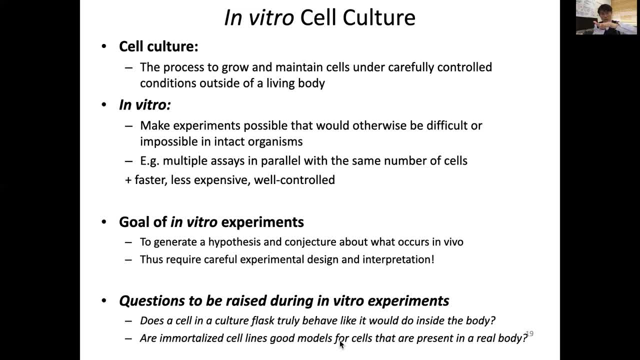 becomes transformed into growth in a plastic petri dish and it's immortalized. so we perform many experiments, for example testing a new drug, anti-cancer drug, with this cell line. however, we have to know that this cell line only comes from one single patient, while out there there are. 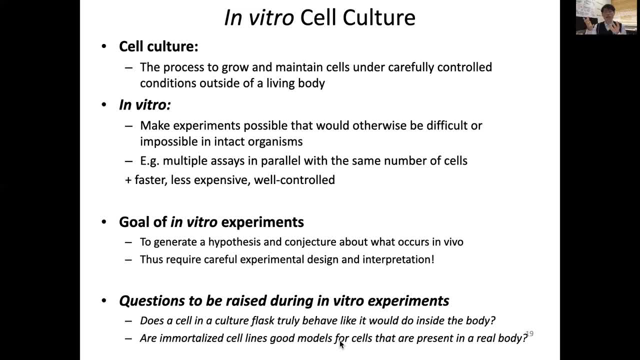 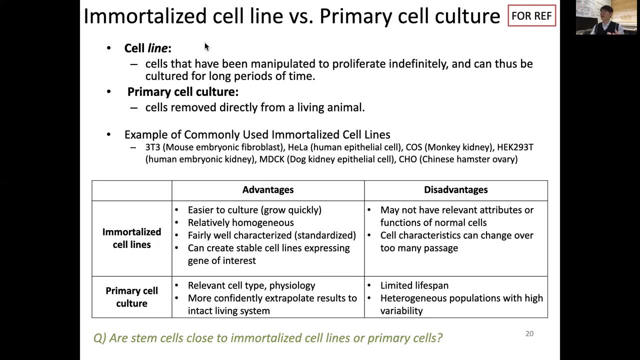 millions of many, many patients whose cancer, even if it's the same, let's say cervical cancer- that may behave not exactly the same. so we have to know the limitation of when we are using a cell line, so that immortalized cell line is one way of in vitro experiments. but there are some. 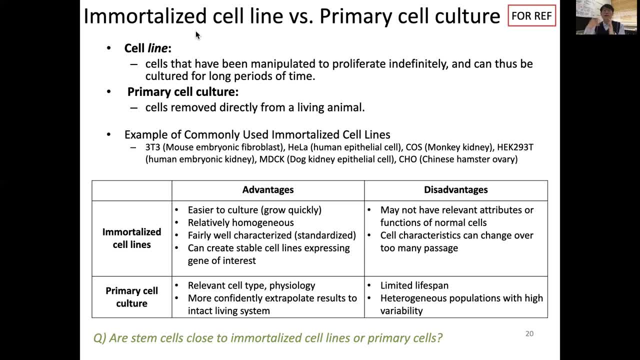 you. in fact, many cell types may not have cell line, which means you have to use a cells coming directly from a living tissue. that we call primary cell culture, and in that case that's also in vitro experiments. but there's a little more different aspect. we should consider so first, when we call cell line, that line. 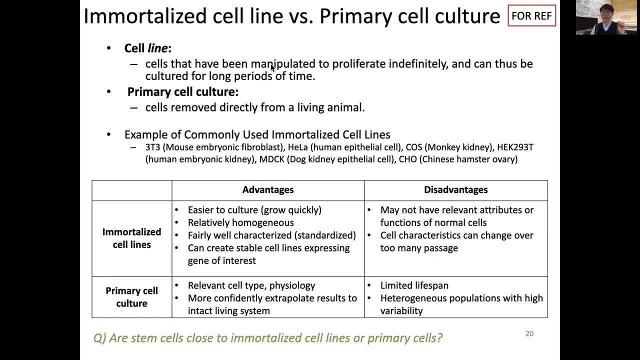 means those cells have been already manipulated to proliferate indefinitely and can does per culture for long period of time, so from one generation to the other generation. so we call it as a passage and it can go as many passages as possible, while primary cell culture coming directly from a living animal usually cannot�� 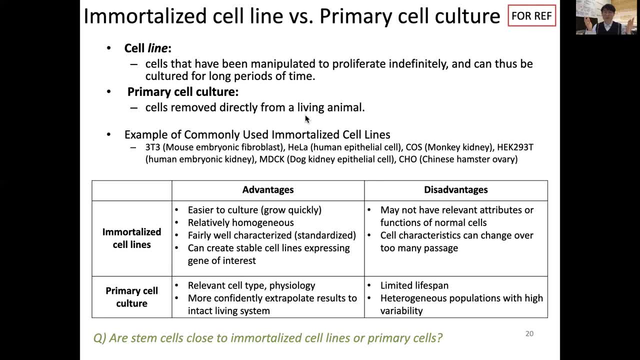 proliferate indefinitely. You remember the telomere? So cells when they divide and divide, there's only a finite number of potential to divide. So that's kind of the limitation of a primary cell culture. So in fact there's not so many cell lines. So there I put some examples of commonly 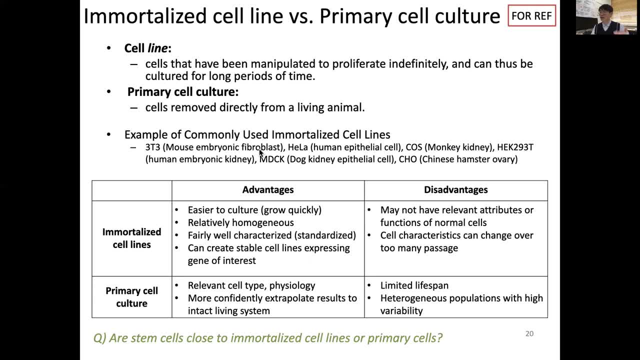 used immortalized cell lines, For example fibroblasts. there's a famous 3T3 cell line, Human epithelial cell. it's a cancer cell named as a HILA cell, or monkey kidney COS cell, or human embryonic kidney HEK cell or dog kidney epithelial cell. 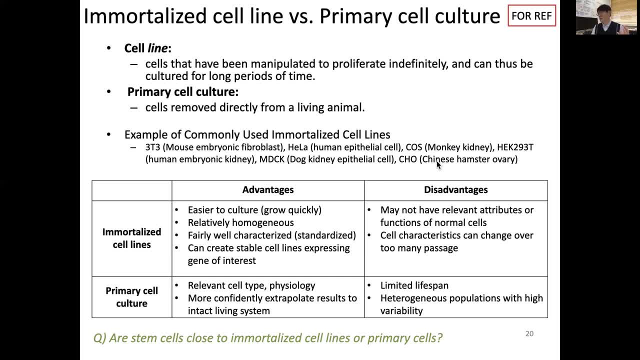 DOCK cell or CHO cell, which is coming from Chinese hamster ovary cell. So there are, like you know, many but still finite number of cell lines established and we use them for different purposes, such as when we want to study breast cancer. then there's a dozens of breast cancer cell line. 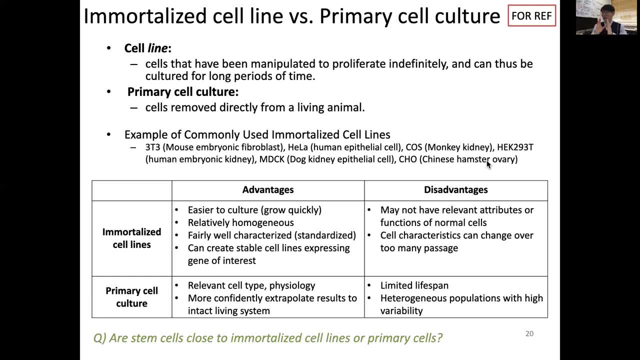 which we want to use. If we want to study, let's say, cellular migration from a wound healing purpose, let's say, we can use 3T3 fibroblast cell line. So they, this way, we have well characterized those cell lines and we can compare from one research, from another. researchers. 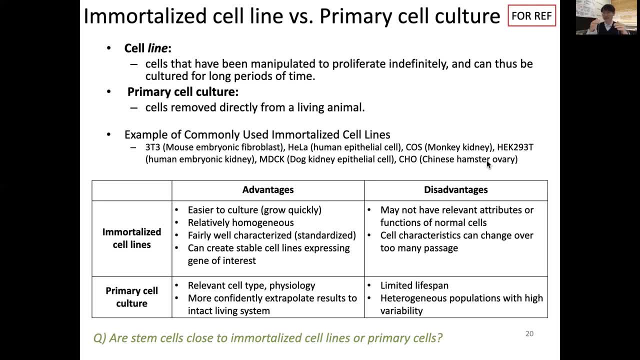 results. So that serves as a good standard. So let me have a table which compares immortalized cell lines and primary cell cultures. So the advantage of immortalized cell line is it's easier to culture because those cell lines are more sensitive to the body than the body. 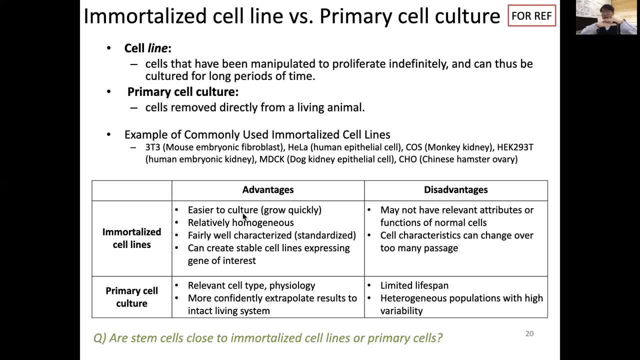 So we can see that there are more genetic differences between the original and the primary cell. so we can see that the primary cell can be more sensitive to the body. like these are very sensitive to the body and that's why it's very easy to use. 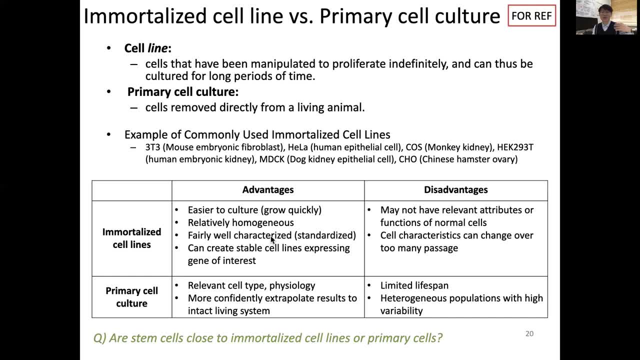 Another benefit of immortalized cell lines is that the cells are already transformed, which means it already adapt itself into a well uh controlled plastic, petri dish environment, big amount. that means we can also manipulate their genes easily so we can create stable cell lines expressing gene of interest. so by using trans genes or overly expressing, or even knock down. 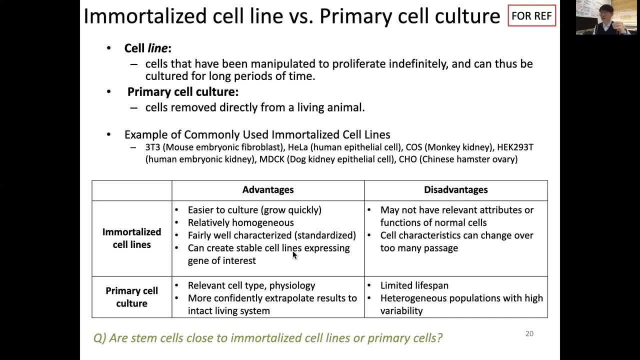 the some of the genes of our interest or not, in compare. in comparison, primary cell culture is supposedly more relevant cell type because it's freshly taken out of the body. so it, though it's more relevant in terms of physiology and, however, the homogeneous aspect, because primary tissue 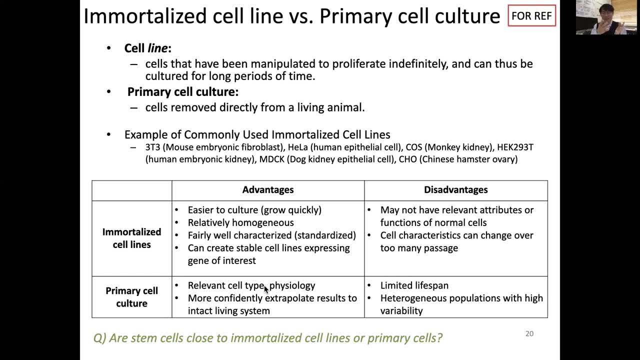 composes or is composed of many different cell types. sometimes it's not as homogeneous when we are using primary cell culture, however, given the primary cell culture it's. the primary cells are from primary cell culture to primary cell culture to primary cell culture to primary cell culture. 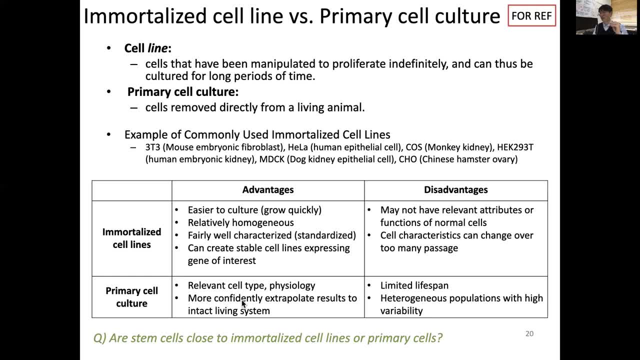 original living tissue, we can have more confidence extrapolating those results to intact living systems, such as going towards in vivo interpretation. so what are the disadvantages of primary cell culture? because you took out from the tissue, it's not well characterized, the lifespan is not indefinite, so it has a limited lifespan, such as if you take out cells. 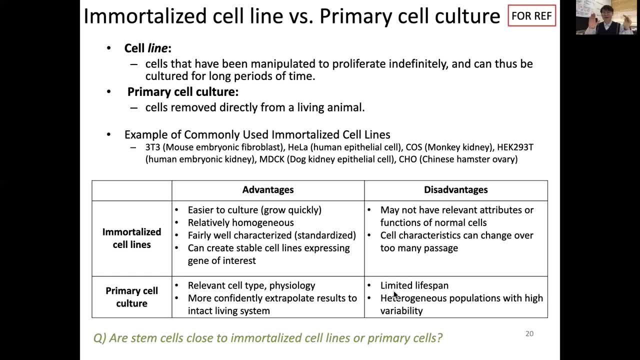 from the tissue, you may not have a long time to perform your experiments, and also heterogeneous population with high variability. so it may be more difficult to prove something with the primary cell culture, while immortalized cell lines may not have the relevant attributes or functions of normal cells, because it's already quite strange cell. and and another thing is, even if let's say 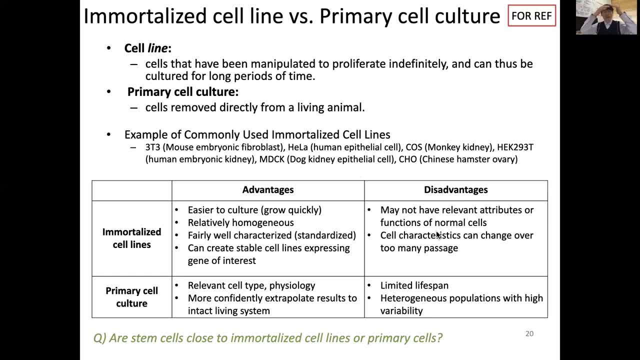 the same heterogeneous cell lines are not the same as the primary cell culture, then it's not true, because what you're seeing is we are not actually really a single cell. that we have a single cell. we are not a single cell. that is the main human, human problems, and we don't. 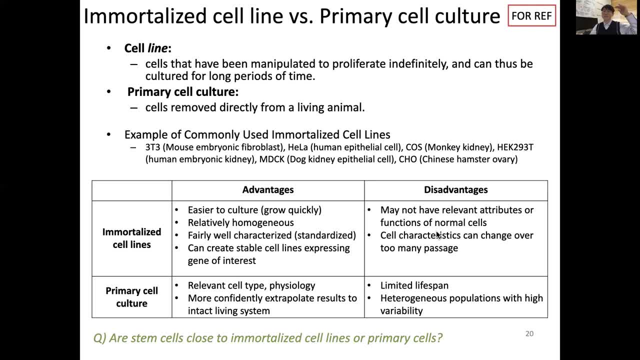 have the same department but, as I mentioned earlier, we don't have the same similar cell structures for the same individuals. so what I want to say is that the general population currently is not the same, but it's not true. so the general population is not important. the general population is not an integral part of human life and it's not an integral 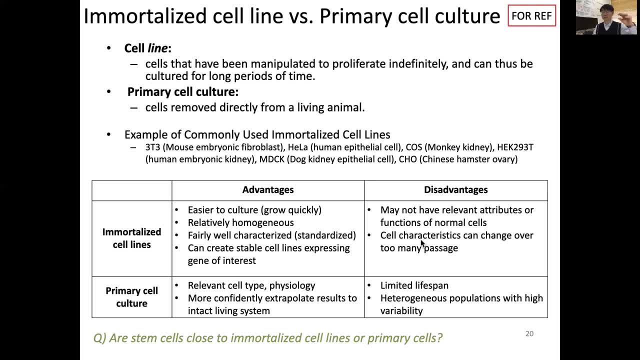 part of human life, but it is the basic thing. the, the general population is important to all living living persons on the plant. that's why highly desirable and particularly interesting of over too many passages. the cells may have adapted or changed its characteristics, So that's possible. So one question we can ask ourselves is: 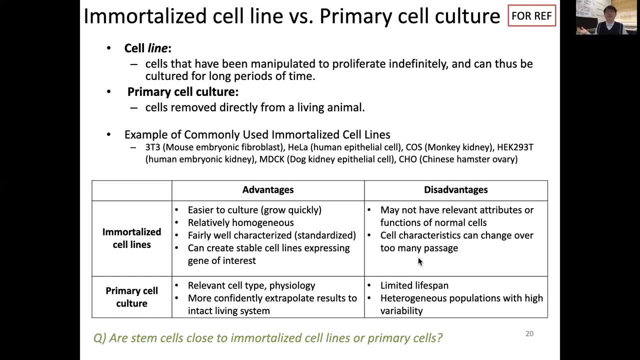 hey, we have learned about stem cells. Are stem cells closed, immortalized cell lines or primary cell culture, Which is an interesting question to ask ourselves? First of all, stem cells usually are coming from an animal. It's in vivo, so it's much like a primary cell. On the other hand, stem cells 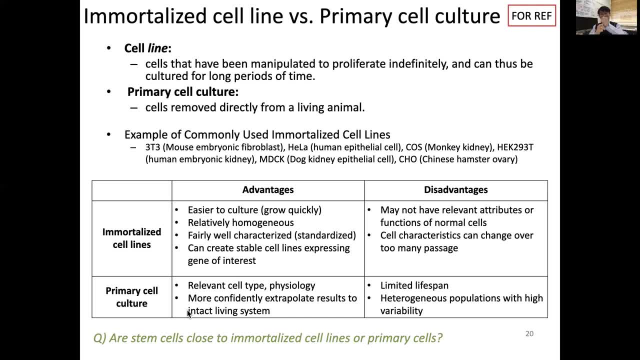 itself has an indefinite self-renewing capability that actually mimics our immortalized cell lines. One of the proofs that the cells that have this stem cell culture is whether they can keep growing or proliferate. to grow home bring a tumor formation called keratoma. So that is one evidence. hey, this is a. 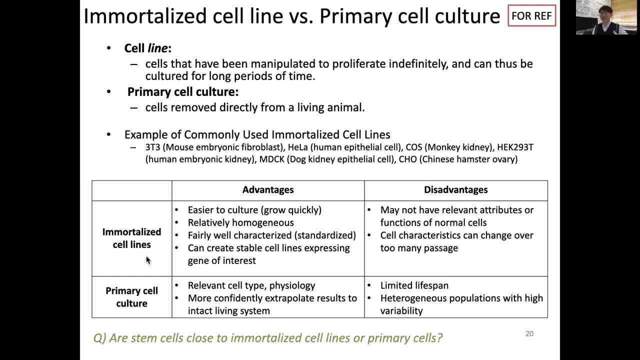 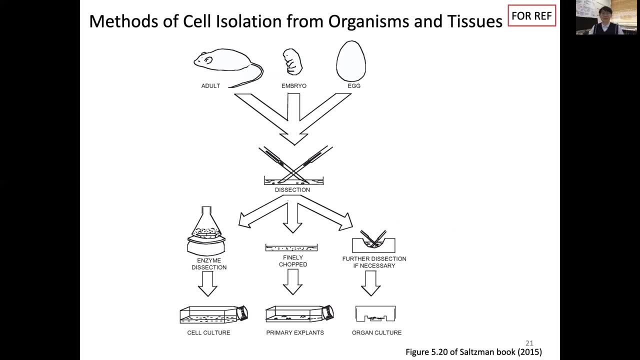 real stem cell. So in that aspect it actually also mimics immortalized cell lines. So how to isolate cells from organisms and tissues? There are a number of ways. I just want to explain with this picture. So our tissue may come from an adult animal, or embryo, or even egg. So we put them into our petri dish. 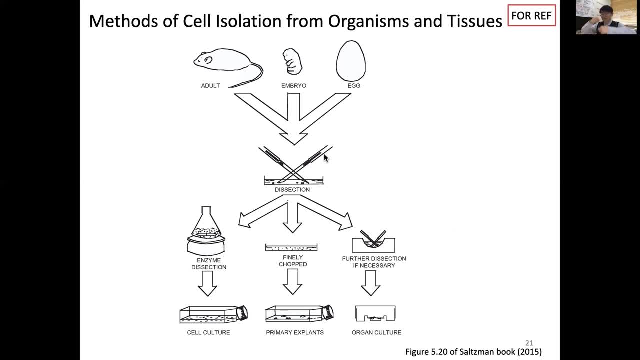 and using a blade to dissect them out. But still, you know, our ways of dissection might be too coarse that we could use either enzyme to digest, So using enzyme to dissect them, and then we can have a cell culture, Or very fine. 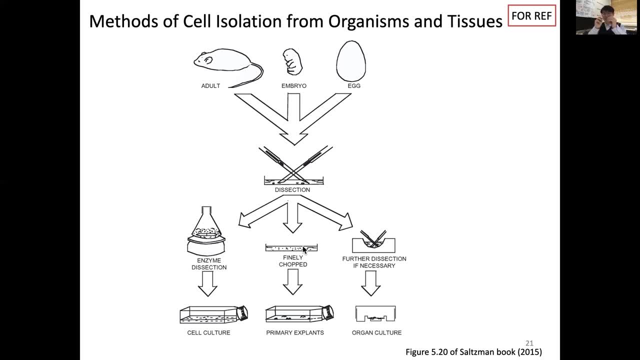 chopping, maybe steel. it's kind of small explant of tissue and that we can actually culture like primary explant Or further dissection. if we need, then we can have a small tissue and we call it as even organ culture. So there are various. 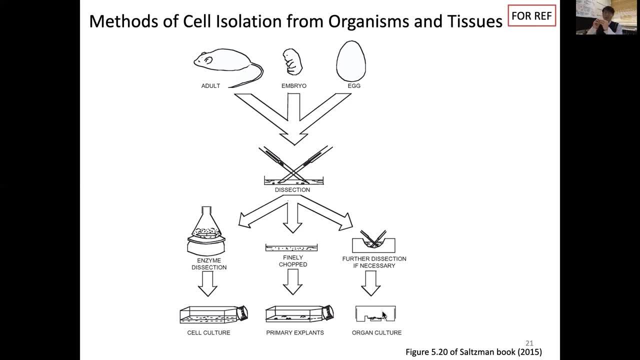 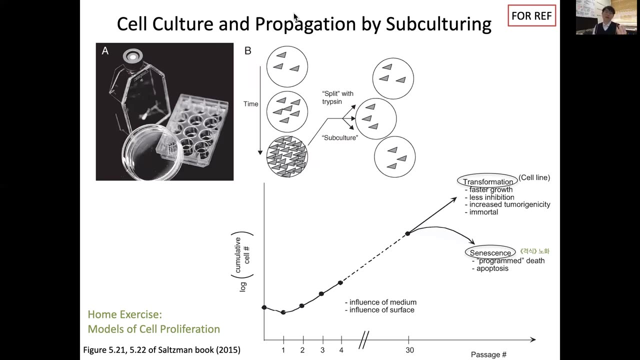 methods of cell isolation, depending on whether we are having a tissue chunk or even disintegrate them into into an isolated cells by using use of enzymes. So when we are culturing cells, the goal is: you grow the cells so that we can do experiment with it, or with that we can actually extract RNA. 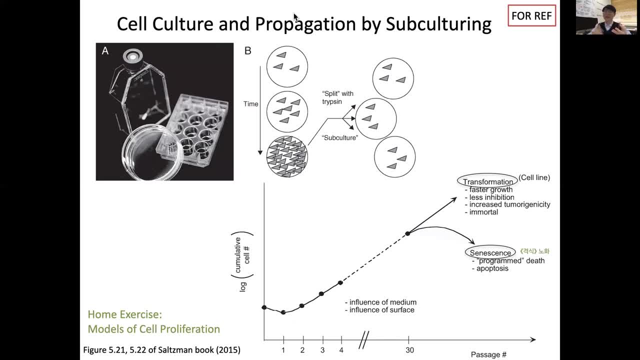 DNA or proteins, and for that we have to use cell culture and we have to grow cells So that we call propagation by subculturing, subculturing. So that's you can see here. So first we put the cells over here and then over time it grows. 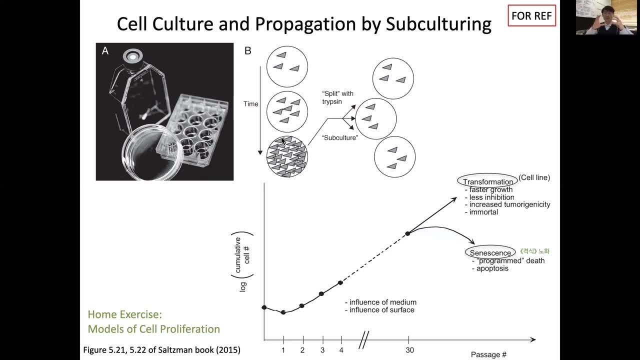 and once it reaches to certain limit, then we actually subculture, meaning that where we took out the cell and we split and from one dish into a number, for example like three, So that's subculture and we run this one again so that we can. 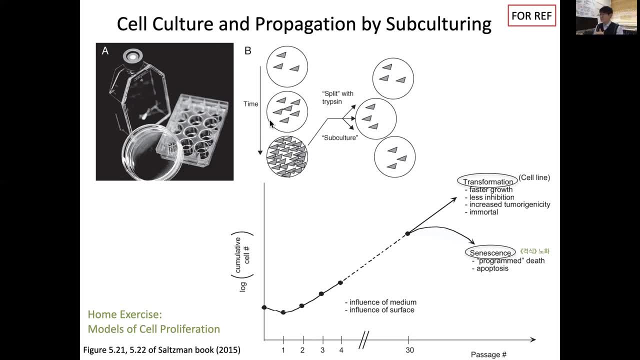 exponentially grow the number of cells. So So. So here is an interesting chart, with x-axis is number of passages from one generation to the next generation and y-axis is a log of cumulative cell number. Because you think about it, cells divide the one to two, two become 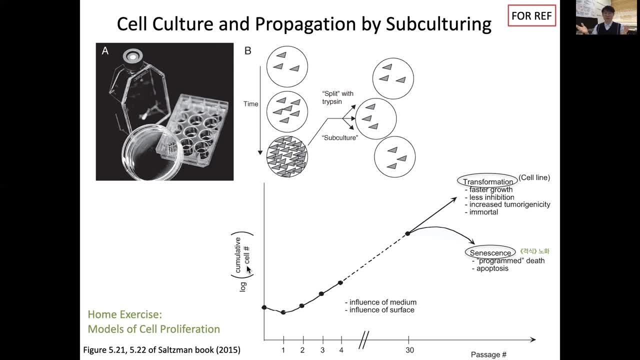 four, so it actually undergoes an exponential growth. So when you plot it in a log plot it will make a kind of a linear graph. So how do we do it? However, you look at this interesting single passage: one, two, three, four- the in the middle is a kind of a dotted line because it's assuming that it can be affected by environment. 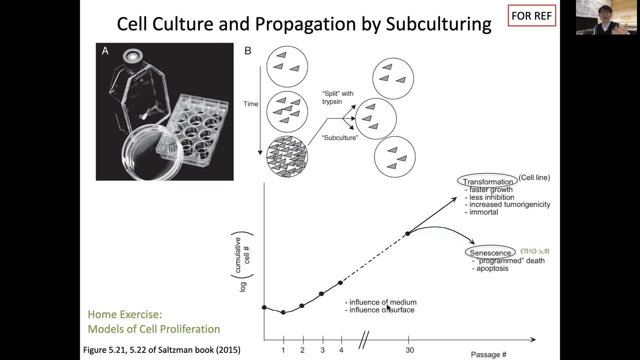 So, for example, influence of medium- are there enough nutrients keep coming? or influence of surface, the surface property. for example, the cells have a contact inhibition property. So normal cells, typically our cells, like to attach to some surface, So that's what we call. 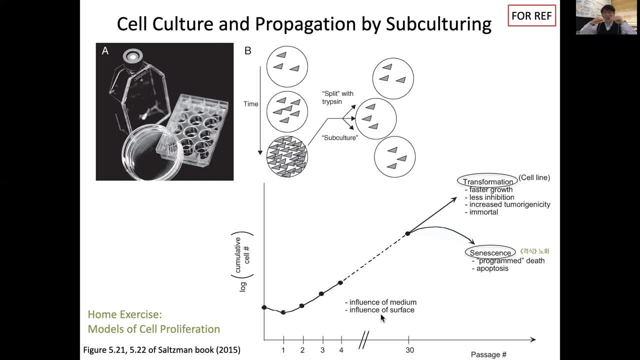 increased dependence And if the cells grow too much to spread out to touch itself, they develop contact inhibition. So those can affect this exponential growth. But during this growth, at some point when the crisis can happen, which means the cells even originating from primary can be transformed into. 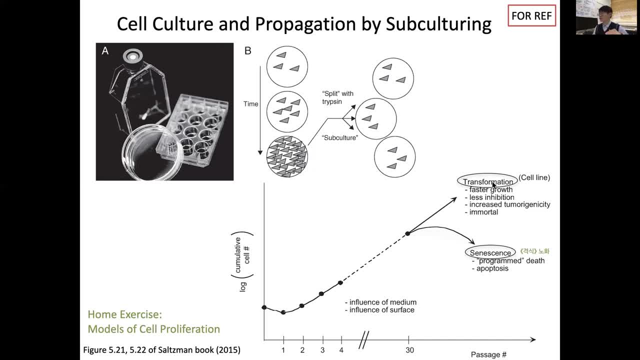 an immortalized cell, So that we call as a transformation, And those are the cells we are using as a cell line. So they typically have a characteristic of faster growth and less contact inhibition And they're likely to generate tumor- tumor, So tumorigenicity- So that these cells can be used for tumor. 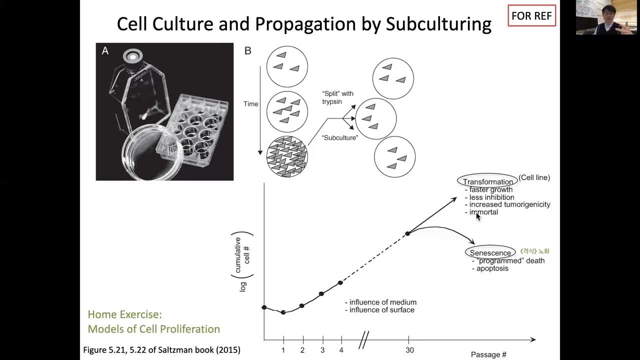 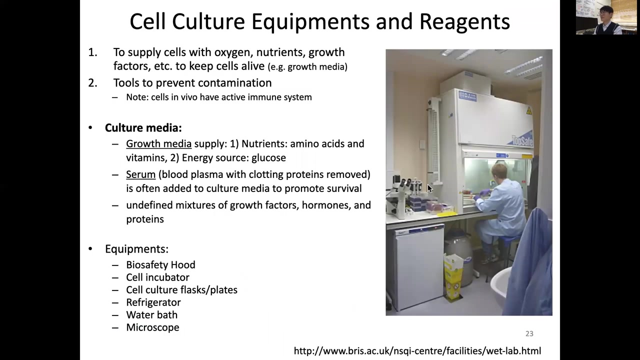 model, in animal or in vivo, And they are immortal, which means they don't die over passage. But typical cells, such as primary cells, and mostly they work, sometime they enter into senescence, which means they are already programmed to die apoptosis. So now I want to go a little detail of cell culture equipment. 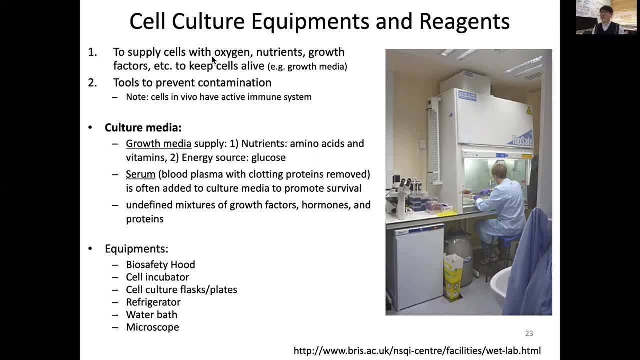 and reagents, So to supply the cells with oxygen, nutrients and growth factors. to keep the cells alive, we need to have a growth media And also we need an environment or equipment to prevent contamination, Because ourselves, like animals, we have an active immune system that there 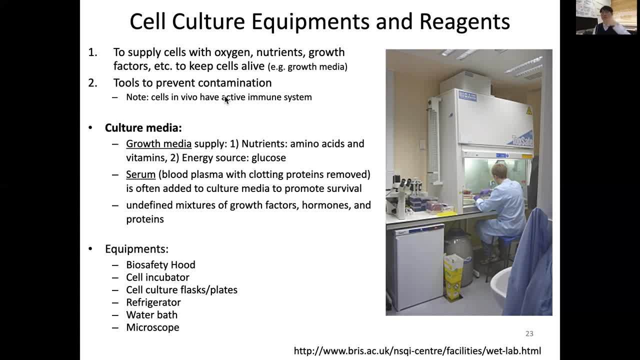 are always bacteria getting into our mouth or our body And we still are okay because we are keep having defense system. But the cell itself has no such a such a system. So we have to be very careful, though those cells are not contaminated. 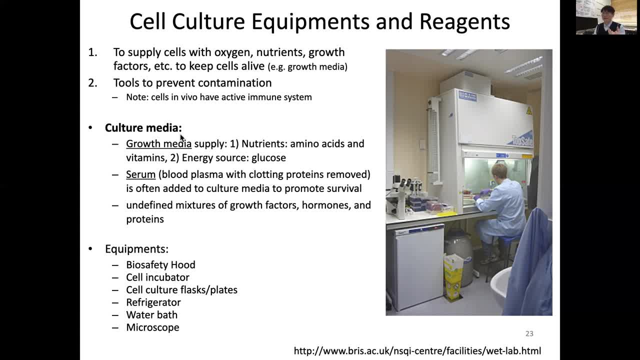 So especially the cells are in the culture media which contains growth media supply, which has nutrients, amino acids and vitamins, and energy source as glucose. So it's also good for if there's even bacteria gets in, they will love to grow here And also we add. 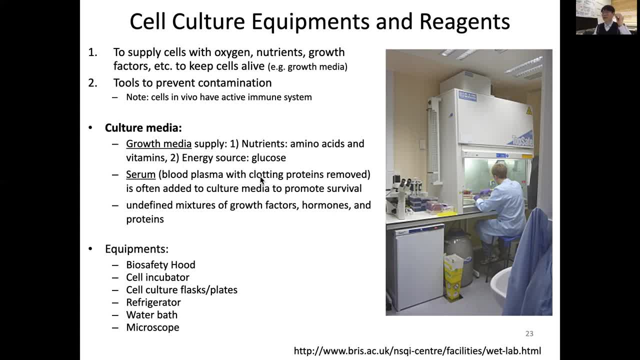 some serum, which is a blood plasma with clotting factors, are removed, So such as BCS, bovine serum, So that is often added, such as 10% into the growth media to culture media. usually they contain a lot of growth factors, So that can promote survivor. However, one thing we have: 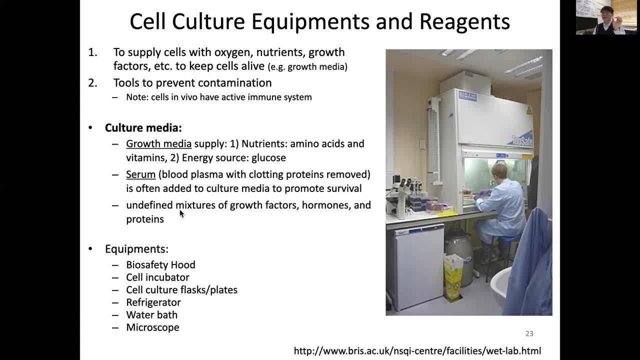 to remember is those serums in fact contains undefined mixtures of growth factors and hormones and protein. So they are good, But sometimes we have to be careful the use of serum when we have to identify a subtle growth comparison because of this unknown effect. So 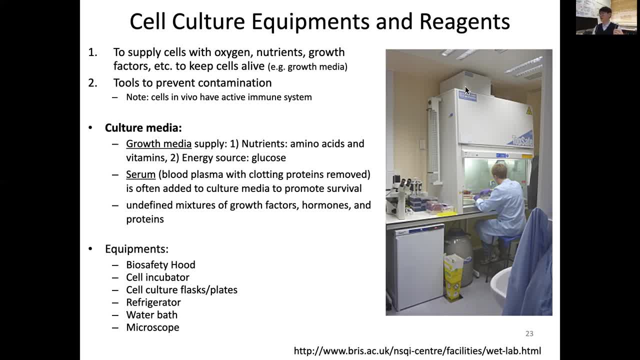 typical cell culture room looks like this And you can see this is called a biosafety hood and or laminar hood, which there's a filter here, and then the wind is coming, already, coming from inside to outside so that it blocks bacteria, And this is called cell incubator, which keeps the cells when you incubate the cell, so it keeps. 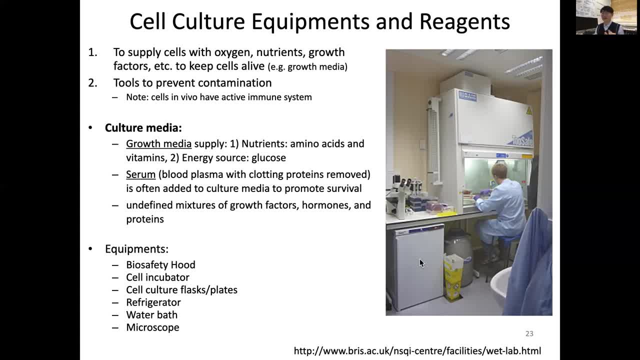 humidity and oxygen and CO2 concentration And you can see some of the cell culture flasks And there it's not there but as a refrigerator because a four degree is very low temperature which keeps down the metabolism. So when we are manipulating the cells and the water bath to warm up the cells and microscope to be able to see the cells, 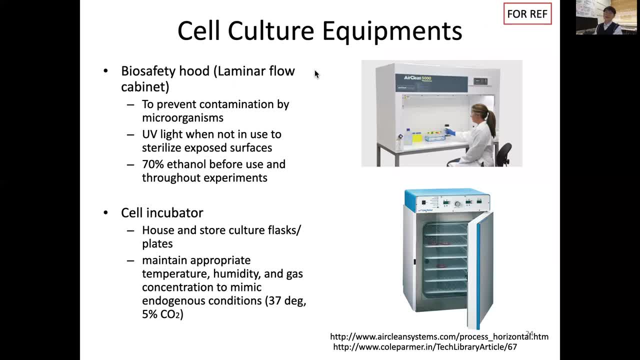 So let's go over one by one. This biosafety hood, or laminar flow cabinet, is to prevent contamination by microorganisms. So it's always blowing in inside to outside And also there's a UV light. So when we are not using, always turn on UV light. 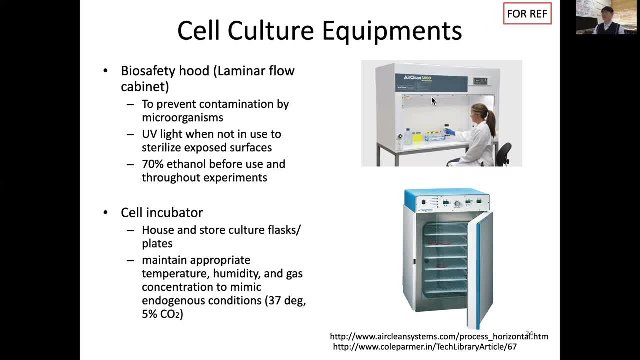 And also there's a UV light. So when we are not using, always turn on UV light. So when we are not using, always turn on UV light, And it's valuable for health And it's valuable for betterơi, and also before and after we are going to use 70% ethanol. 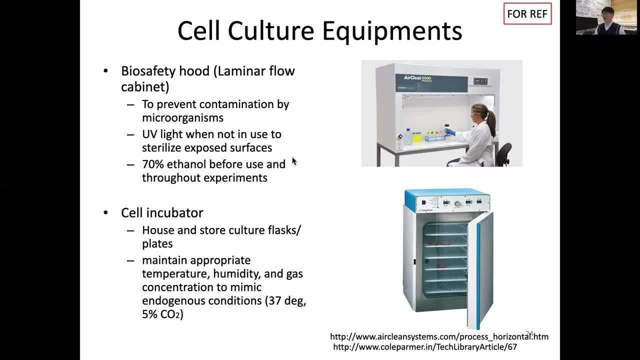 and also before and after we are going to use 70% ethanol, and also before and after we are going to use 70% ethanol, So that you know, clean up the surface For for preventing any contamination to and SED incubator looks like this: It's small housing and looks like there's a plate and underneath their water. which warms up and keeps the humidity. which warms up and keeps the humidity. So how sensitive cultural flasks or plate? So how sensitive cultural flasks or plate? I know this is something I've been done a lot, so I don't know if it's gonna happen. 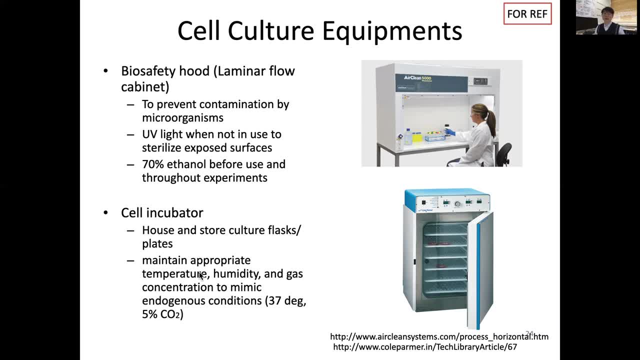 I know this is something I've been done a lot, so I don't know if it's gonna happen. flasks or plates and we have to maintain appropriate temperature, typically 36.5 degree, and humidity and gas concentration to mimic endogenous conditions so that keep 37 degree and co2 concentration as a 5%, also cell. 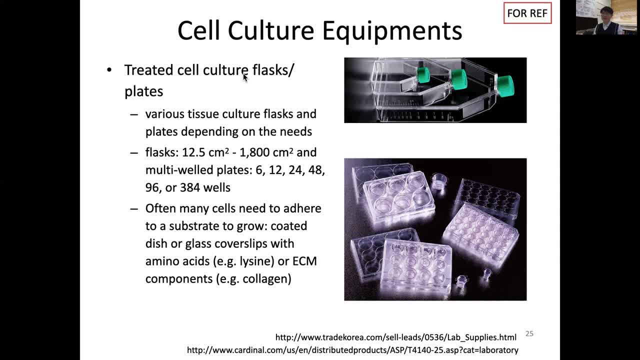 culture, we are using cell culture flask. there are different kinds of flask. one example with a size depending on our needs- so these are called so-called tea flask- and depending on the area of the bottom and we can have 12.5 until like 1800 and also so this is good for like growing the cells, especially like 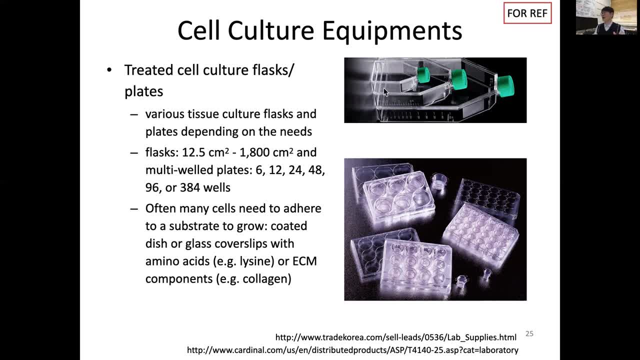 tumors we can use even like 225 cubic square centimeter so that we can grow like 10 million cells easily, while for precise assay or precise comparison of treatment versus control, we may want to use multi-welded cell plates. so you can see here six well plate or 12 well plate, 24 well plate or 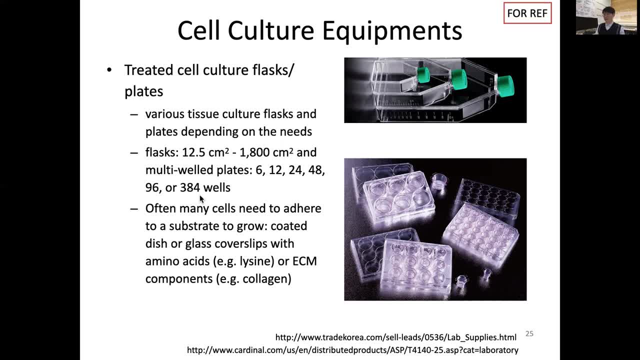 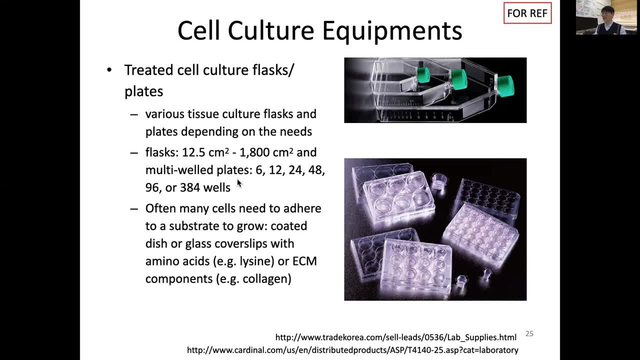 multiple experiment simultaneously so that we can get more statistically meaningful and reproducible results. often many cells need to adhere to a substrate growth, so it depends on cell from cell to cell. so sometimes we have to coat the dish or glass cover slip with amino acids such as lysine or 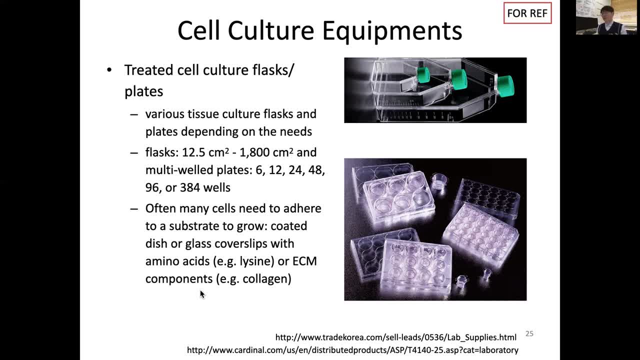 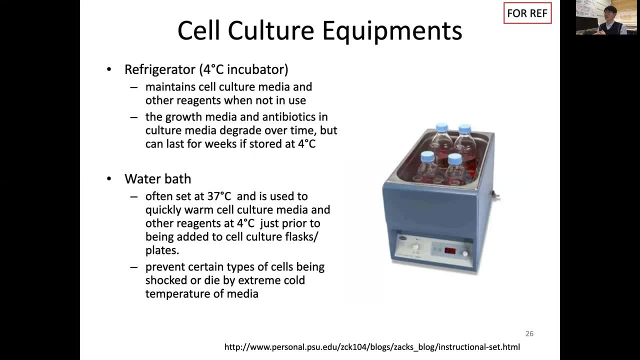 extracellular component- collagen or laminin for a specific cell growth, and many times the reagents. we are keeping it in the refrigerator or fridge, which is four degree incubator, to keep the cell culture media and other reagents when not used, like we are keeping our food in the refrigerator and the growth media. 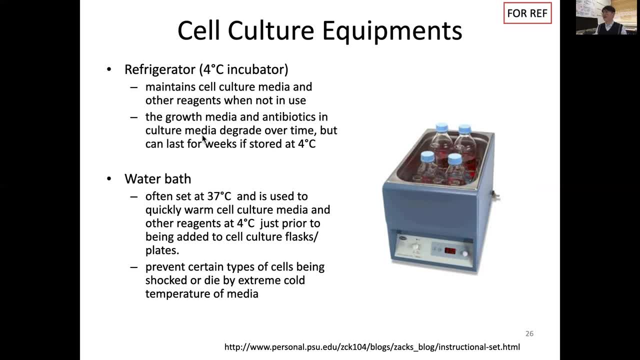 and antibiotic in culture media. of course we are keeping our food in the refrigerator and the growth media and antibiotic in culture media. of course we are keeping our food in the refrigerator. and the growth media and antibiotic in culture media. of course they contain proteins and they can degrade over. 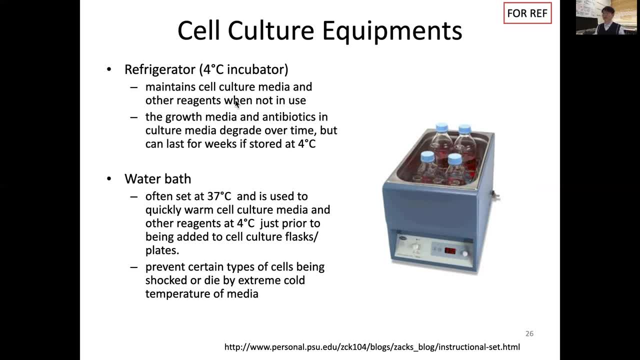 course they contain proteins and they can degrade over course they contain proteins and they can degrade over time, but they can last for weeks if stored in time. but they can last for weeks if stored in time, but they can last for weeks if stored in the refrigerator. also, water bath often. 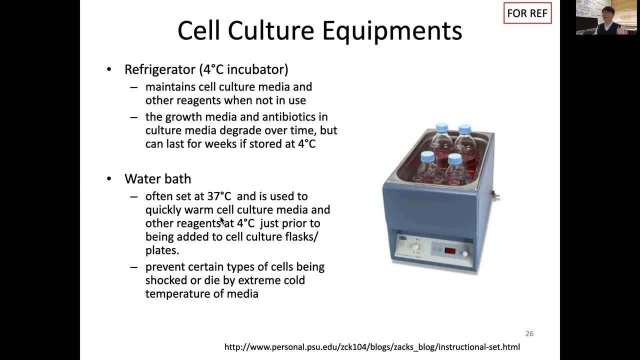 the refrigerator also water bath. often the refrigerator also water bath. often set at 37 degree. it's to quickly warm. set at 37 degree, it's to quickly warm. set at 37 degree, it's to quickly warm. cell culture media and other reagents. cell culture media and other reagents. 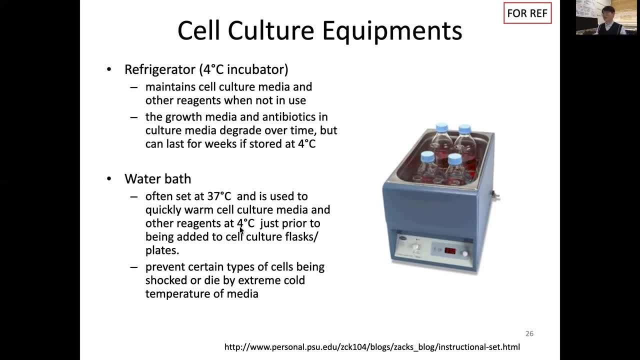 cell culture, media and other reagents when they directly come in contact with, when they directly come in contact with, when they directly come in contact with the cells. so, however, in many times, the cells. so, however, in many times, the cells. so, however, in many times, cancer cells are so strong that I, you 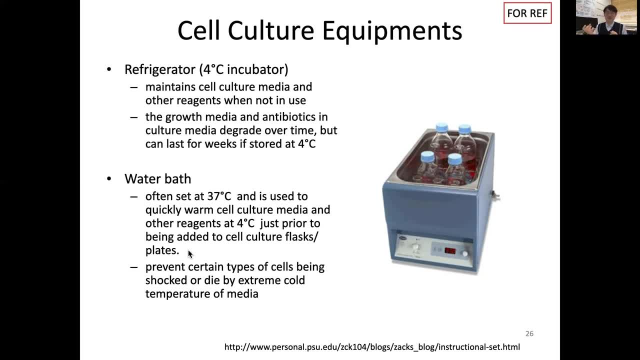 cancer cells are so strong that I, you cancer cells are so strong that I, you know. many people found we don't even need know. many people found we don't even need know. many people found we don't even need to warm up the growth meter. still, the. 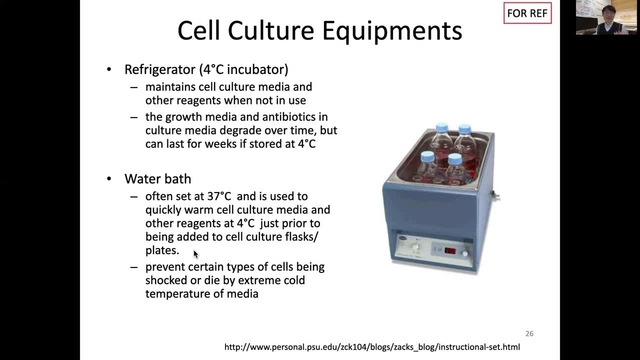 to warm up the growth meter- still the. to warm up the growth media- still the cancer cells can survive very well, but cancer cells can survive very well. but cancer cells can survive very well. but you know it depends on your experiments. you know it depends on your experiments. 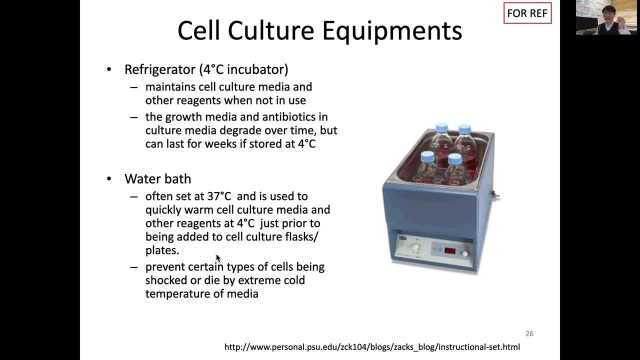 you know, it depends on your experiments. so let's say if you are interested in. so let's say if you are interested in. so let's say if you are interested in. and the cells are so precious, such as a, and the cells are so precious, such as a. 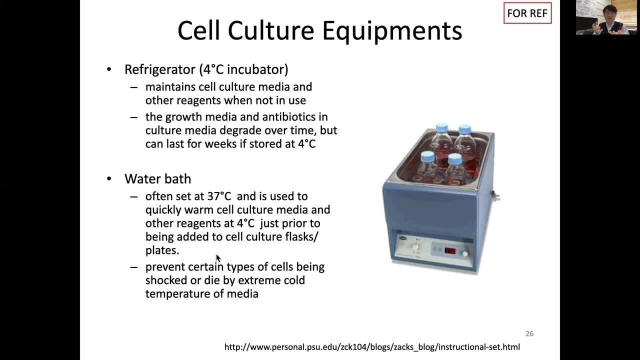 and the cells are so precious, such as a primary cell, the numbers are so small. primary cell, the numbers are so small. primary cell, the numbers are so small that you don't want to lose them. because that you don't want to lose them, because that you don't want to lose them because of this cold water, then cold culture. 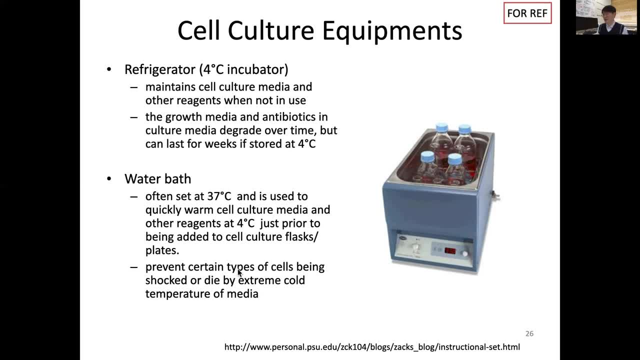 of this cold water, then cold culture. of this cold water, then cold culture. media, then you have to warm them up. so media, then you have to warm them up. so media, then you have to warm them up so it prevents certain type of cells being. it prevents certain type of cells being. 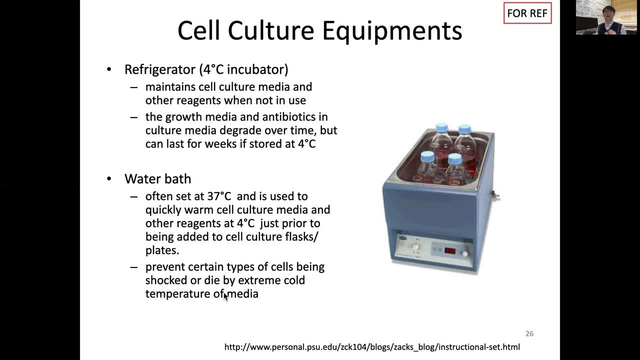 it prevents certain type of cells being shocked or died by extreme cold. shocked or died by extreme cold, shocked or died by extreme cold. temperature of media at 4 degree. because temperature of media at 4 degree, because temperature of media at 4 degree because the cells are optimal at our. 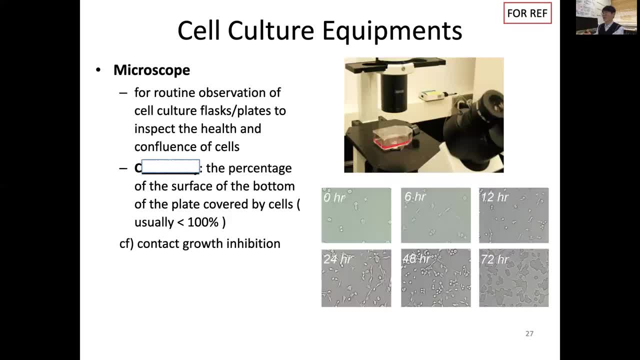 the cells are optimal at our the cells are optimal at our physiological temperature: 37 degree and physiological temperature 37 degree and physiological temperature 37 degree. and once you are doing this, you have to, once you are doing this, you have to, once you are doing this, you have to watch the cell, whether how the cells 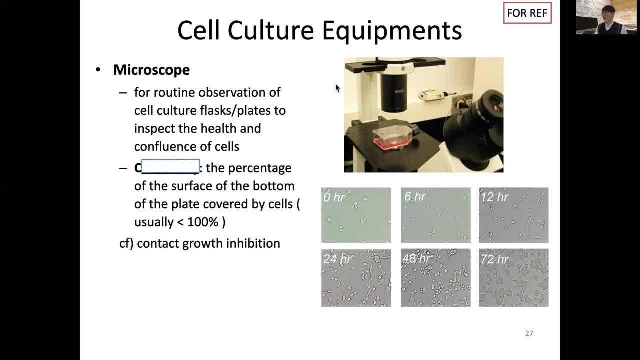 watch the cell, whether how the cells watch the cell, whether how the cells grow, so for routine, like every day, or grow so for routine, like every day, or grow so for routine, like every day or every other day, for microscope provides every other day, for microscope provides every other day. for microscope provides an routine observation of cell culture. 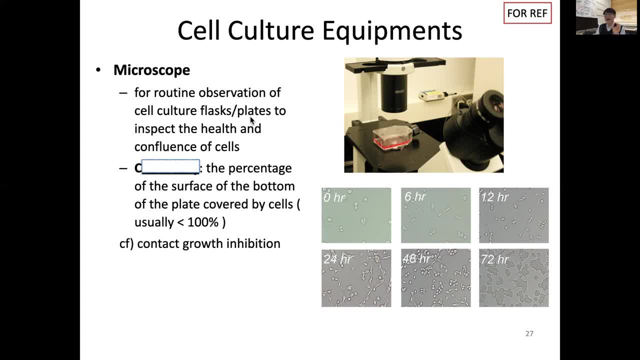 an routine observation of cell culture. an routine observation of cell culture. flasks or plates to inspect the health. flasks or plates to inspect the health. flasks or plates to inspect the health and confluence of self confluence or and confluence of self confluence, or. 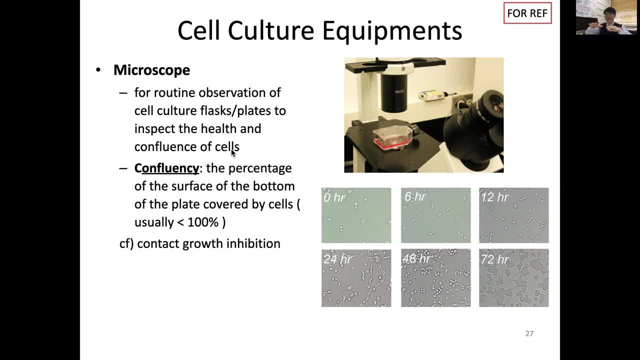 and confluence of self confluence or confluence C means how much coverage. the confluence C means how much coverage. the confluence C means how much coverage the cells on the on the plate, so the cells on the on the plate. so the cells on the on the plate, so the percentage of the surface of the bottom. 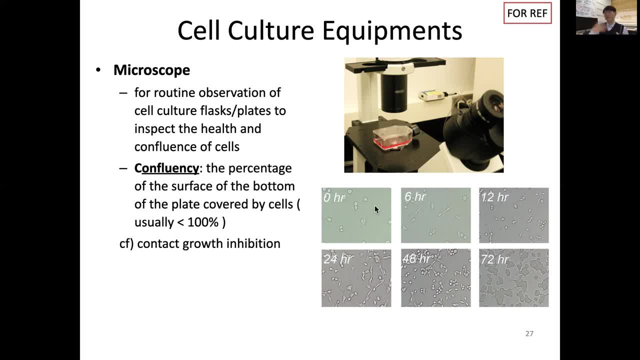 percentage of the surface of the bottom, percentage of the surface of the bottom of the plate covered by itself. so it's of the plate covered by itself. so it's of the plate covered by itself. so it's from 0 to 100% and you can see this this. 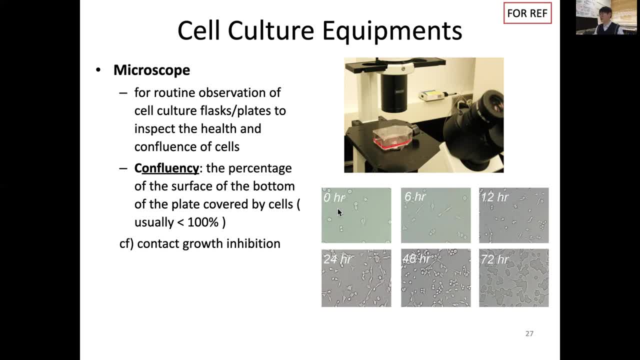 from 0 to 100% and you can see this, this from 0 to 100%, and you can see this, this particular example of T flask. you watch particular example of T flask. you watch particular example of T flask. you watch this and you take pictures of this cell. 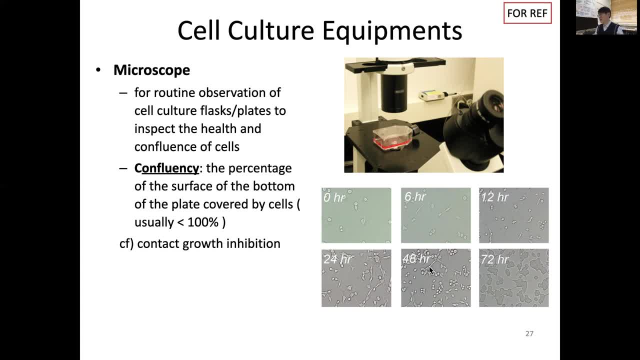 this and you take pictures of this cell. this and you take pictures of this cell growth every like six hours or days. you growth every like six hours or days. you growth every like six hours or days. you can see at 72 hours or three days after. can see at 72 hours or three days after. 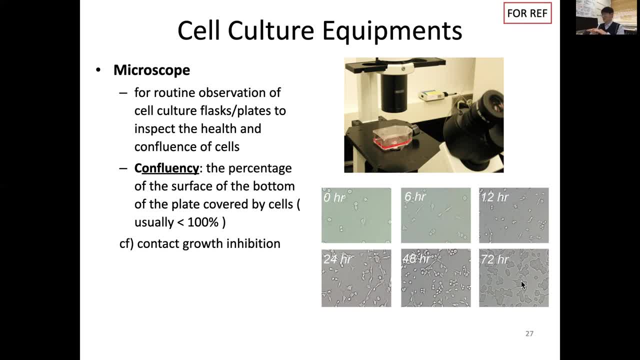 can see at 72 hours or three days after the cells form and attach them. so this the cells form and attach them. so this the cells form and attach them. so this: when they start to attach and grow they. when they start to attach and grow they. when they start to attach and grow, they may slow down due to contact inhibition. 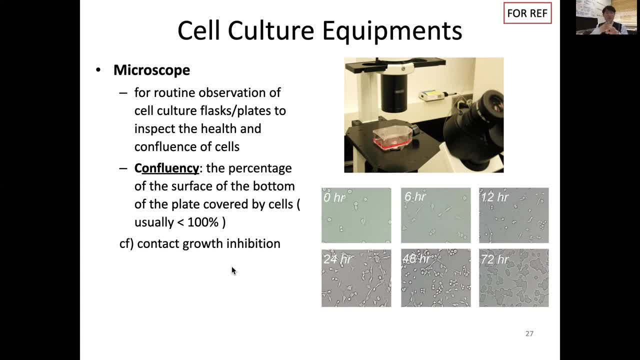 may slow down due to contact inhibition. may slow down due to contact inhibition. but that's giving you an idea that, hey, but that's giving you an idea that, hey, but that's giving you an idea that, hey, it's time to split the cell from one to. 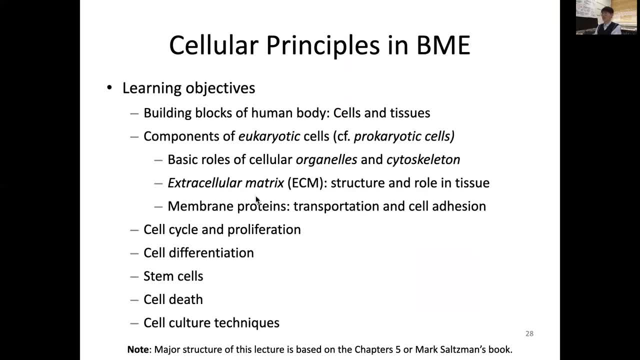 it's time to split the cell from one to. it's time to split the cell from one to like three or multiple dishes. so that like three or multiple dishes. so that like three or multiple dishes, so that you can keep grow. so this ends the you can keep grow. so this ends the. 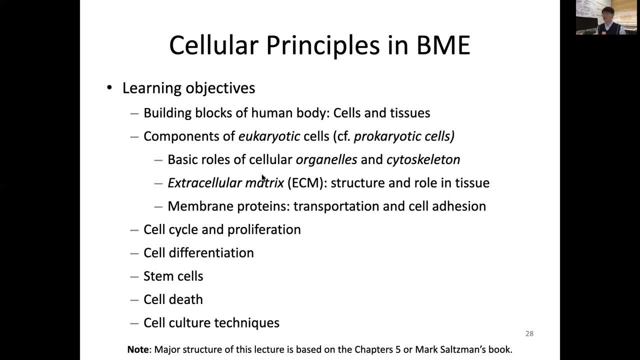 you can keep grow. so this ends the cellular principle. and we've talked cellular principle and we've talked cellular principle and we've talked about building blocks of our human body, about building blocks of our human body, about building blocks of our human body, cells and tissues and components of 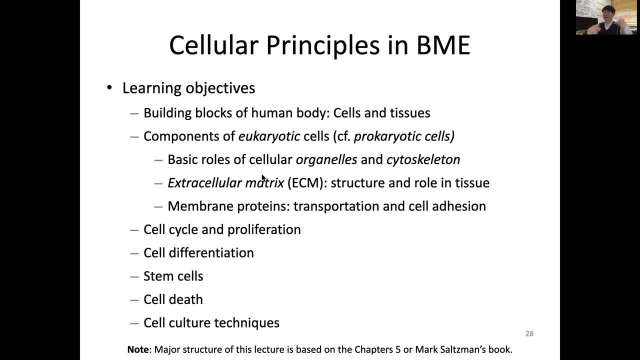 cells and tissues and components of cells and tissues and components of eukaryotic cells and including eukaryotic cells and including eukaryotic cells, and including cytoskeleton extracellular matrix and cytoskeleton extracellular matrix and cytoskeleton extracellular matrix and membrane proteins and the cell cycle. and. 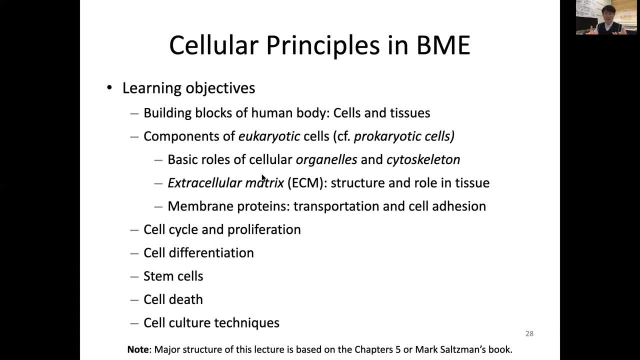 membrane proteins and the cell cycle and membrane proteins and the cell cycle and proliferation and differentiation, especially proliferation and differentiation, especially proliferation and differentiation. especially stem cells were focused because it stem cells were focused, because it stem cells were focused, because it has a big importance in biomedical, has a big importance in biomedical. 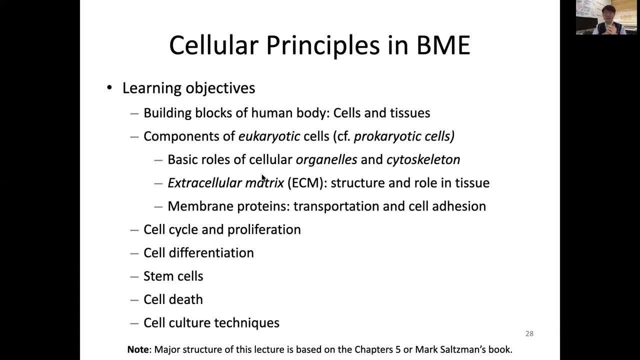 has a big importance in biomedical engineering at the same time, naturally engineering, at the same time, naturally engineering at the same time, naturally occurring cell death and also occurring cell death and also occurring cell death, and also as apoptosis, and we also covered about as apoptosis and we also covered about. 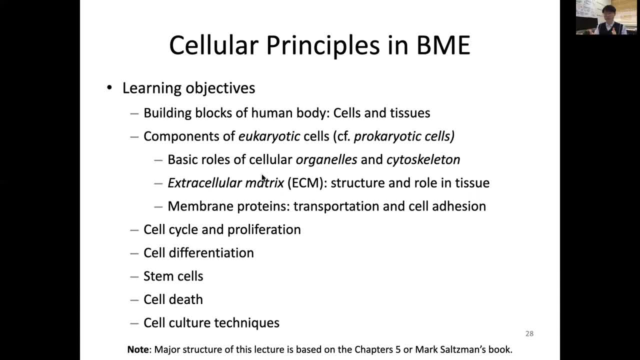 as apoptosis. and we also covered about necrosis, which is necrosis, which is necrosis, which is from the injury or infection, or from the injury or infection, or from the injury or infection, or exogenous ways of cell, premature cell, exogenous ways of cell, premature cell. 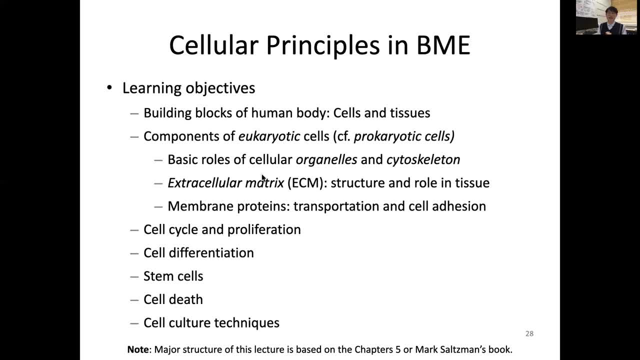 exogenous ways of cell premature cell death and death and death, and the core of this biotechnology depends a. the core of this biotechnology depends a. the core of this biotechnology depends a lot on the development of cell culture. the core of this biotechnology depends a lot on the development of cell culture. 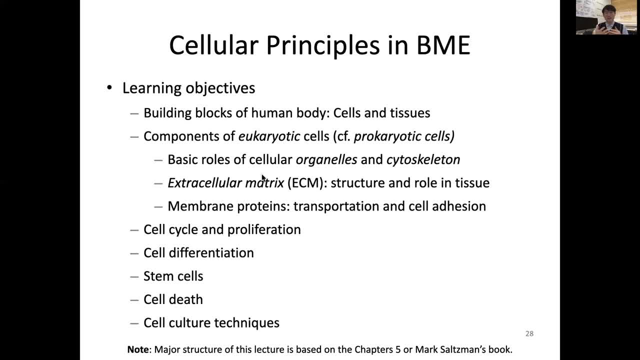 the core of this biotechnology depends a lot on the development of cell culture techniques, techniques, techniques which allows us to grow cells and which allows us to grow cells and which allows us to grow cells and tissues outside of the body, so that we tissues outside of the body, so that we 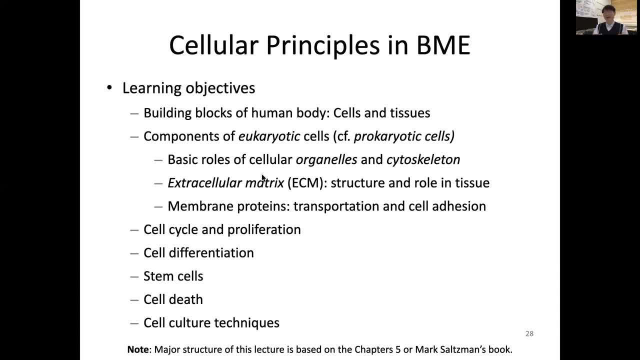 tissues outside of the body so that we can get the material, can get the material, can get the material. in vitro experiments and also a in vitro experiments and also a in vitro experiments and also a biologically relevant study. biologically relevant study. biologically relevant study with enough amount of cells. so thank,